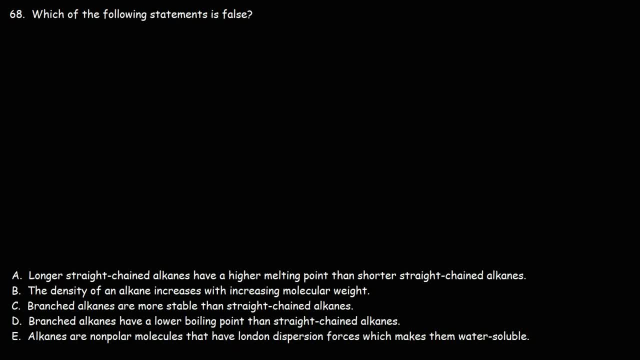 Number 68.. Which of the following statements is false? Now, this problem is basically a review of the physical properties that we've considered regarding alkanes, But let's go through each one. So answer choice. A Longer, straight chained alkanes have a higher melting point than shorter. 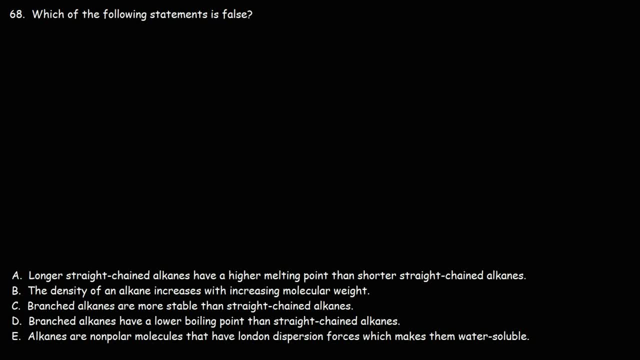 straight chain alkanes. Is that true or false? Well, let's find out. Let's compare pentane with octane. So pentane contains five carbons, Octane contains eight carbon atoms. The melting point of pentane is negative 130 degrees Celsius, and the melting point of octane 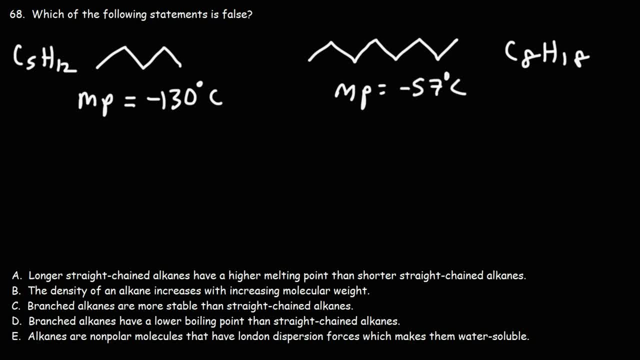 is negative 57 degrees Celsius. So octane has a significantly lower melting point And for one reason it has more van der Waal forces or London dispersion forces acting on it. So A is a true statement: Longer chain alkanes have higher melting points than shorter chain alkanes. 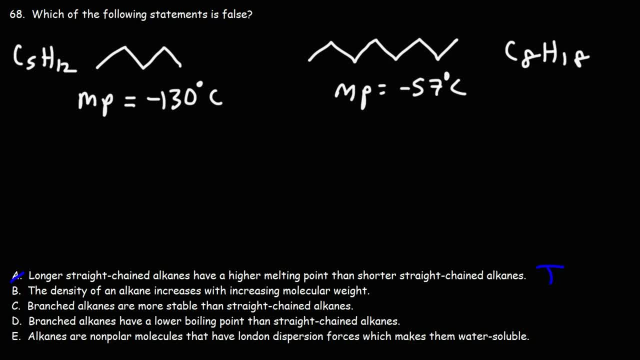 Now, what about B? The density of an alkane increases with increased molecular weight. So what about C? So what about B? The density of an alkane increases with increased molecular weight. So with these two examples, we know that octane has a higher molecular weight than pentane. The density of pentane is 0.63 grams per milliliter. The density of octane is 0.70.. Generally speaking, as the molecular weight increases, the density of the alkane increases as well. So B is also a true statement. 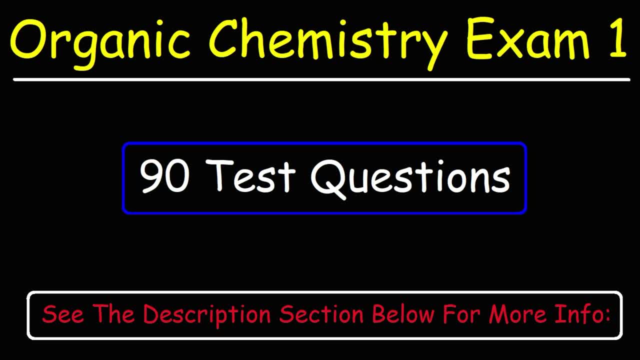 Now I want to take a moment to let you know that the video that you're currently watching only represents one test question out of the 90 questions that are found in my Organic Chemistry 1 Exam 1 video. So for those of you who want access to the full video, check out the links. 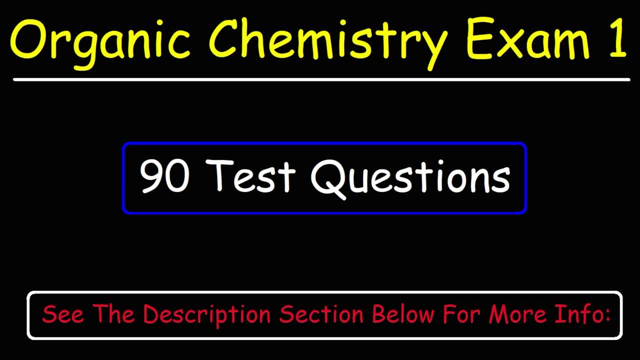 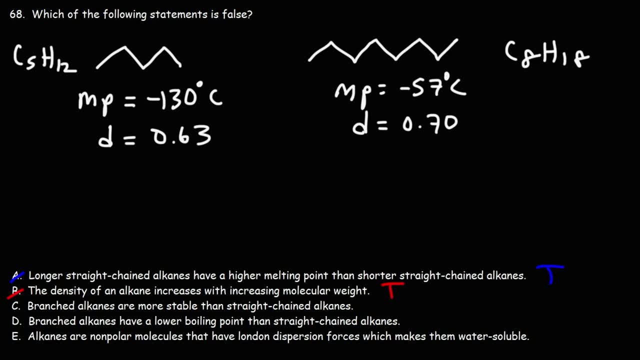 in the description section below this video. Now let's get back to the problem. Now, what about answer choice C? Branch alkanes are more stable than straight chain alkanes. Is that true or false? Well, let's write up an example. 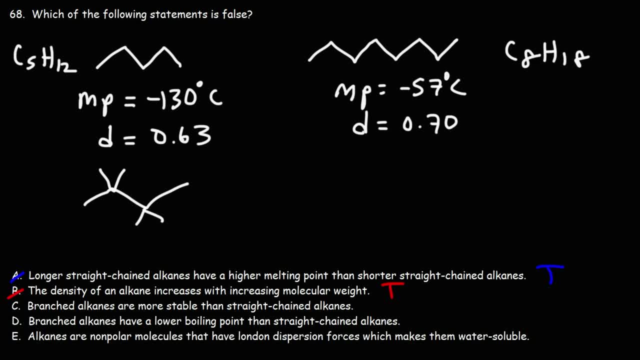 So here we have two, three- I mean two, two, three, three tetra methyl butane, and let's compare that to octane. So both of them have the same chemical formula: 8 carbon atoms, 18 hydrogen atoms. In a previous problem we talked about the heat of combustion for 2, 2, 3, 3 tetra methyl butane. And it was negative 54- 52 kilojoules per mole. but for octane it was negative 54- 70 kilojoules per mole. The alkane with the lower heat of combustion is going to be the one that is second, because it releases less energy when reacting with oxygen in order to 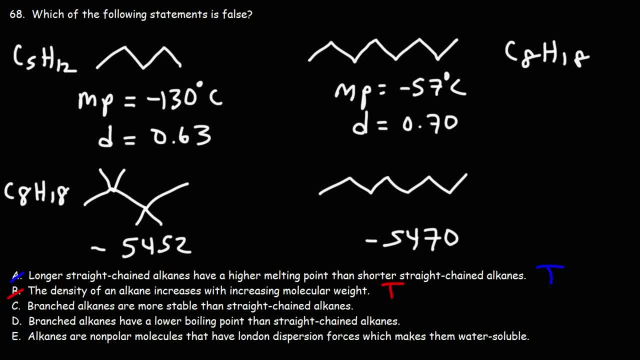 produce carbon dioxide and water. so because the branched alkane has a lower absolute value of the heat of combustion, because the higher the number of potassium carboni and water in the alkyl, the ISO is lower. Therefore, you would need to add another 2 field을- Was it apples- to the one entry. Gotta reduce the number of act concerning 0-2. in case you accidentally need me to be calm If you get a power plug and don't have it on your phone, do consider the questions I'd like to take for you. So just remember the deadline of the video is 24-24-24.. Have a good time. My name is Jaywen Gall and I will let you know what the next question is. Also, please let me know if you have more questions, The best. 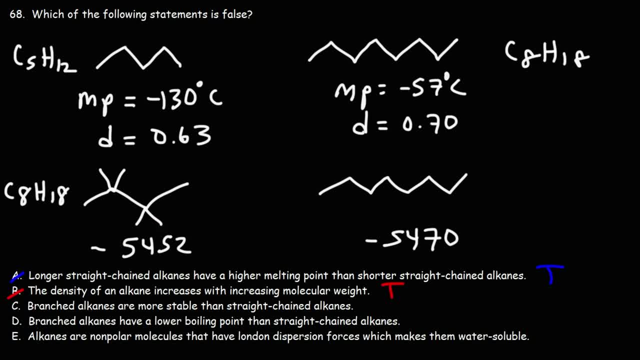 than the straight-chain alkane. we could say that C is a true statement. The heat of combustion tells us which one is more stable, So branch alkanes are indeed more stable than straight-chain alkanes, and the reason is because they have lower heats of combustion. 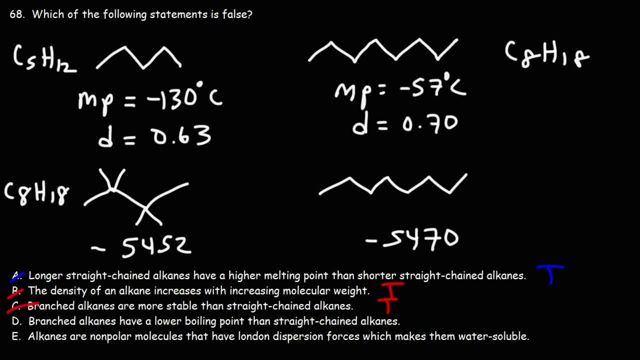 that is, lower absolute value of the heat of combustion. Now, looking at answer choice D, we could say branch alkanes have a lower boiling point than straight-chain alkanes. True or false? Now, this is a true statement When you have a branch alkane. 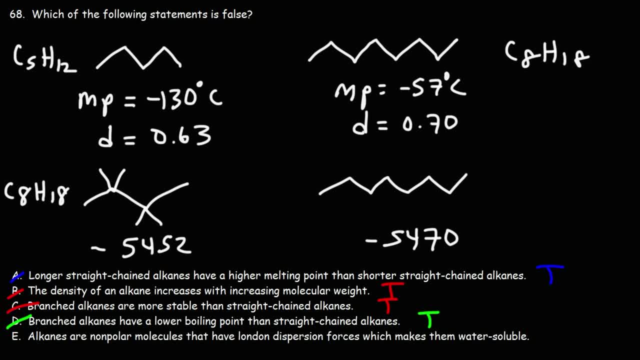 there's going to be less area of contact between adjacent alkane molecules And because of that less area of contact, there's less van der Waal interactions between molecules. So the forces holding them together prevent the formation of a branch alkane And prevent them from boiling off is reduced. 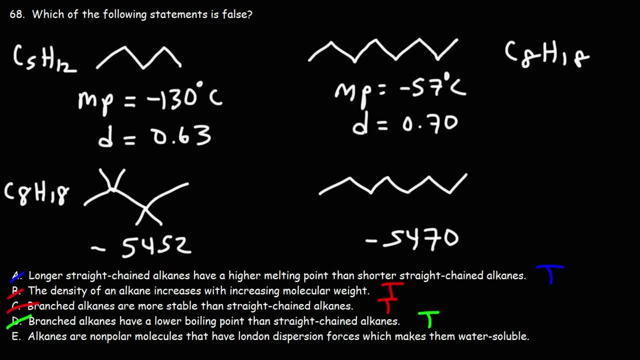 So that's why branch alkanes have a lower boiling point than straight-chain alkanes. The boiling point for 2,2,3,3-tetramethyl butane is 107 degrees Celsius. For octane it's 126 degrees Celsius.